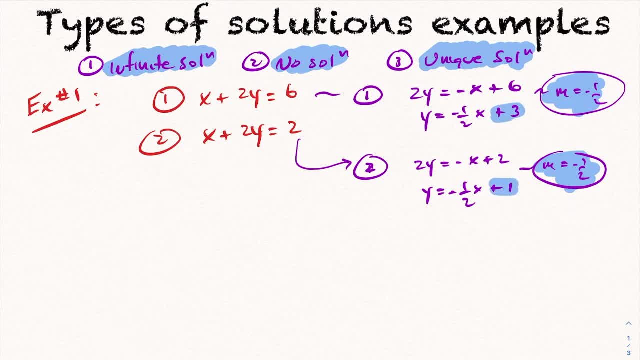 One has a y-intercept of three, the other has a y-intercept of one. So if I go to graph this thing, if I were to do a quick little sketch of this, they're both decreasing, they have negative slopes, but one might look something like this and the other might look something like this. 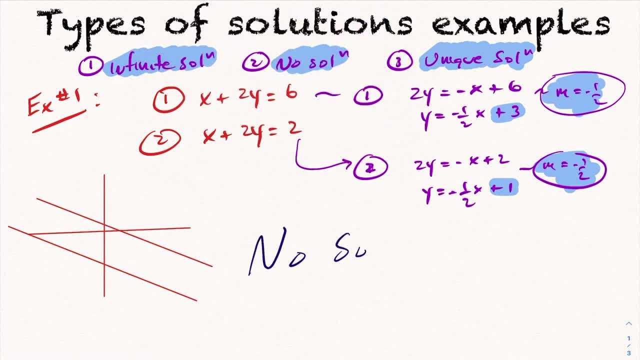 All right. So again, this was overkill. We probably saw it a lot sooner. but the idea here is: there's no solution for this, And the reason for that is the slopes. The lines are parallel, but they have different y-intercepts. 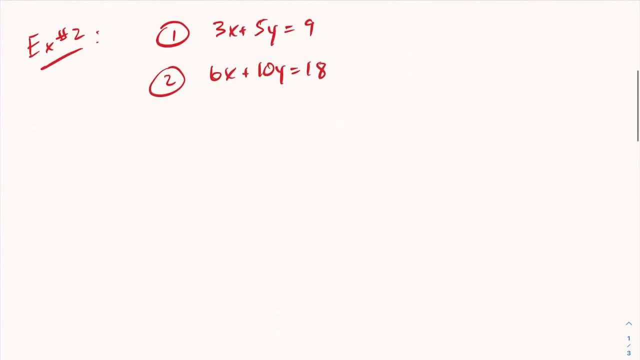 They're not the same equation, All right. Equation 2: here Again, whenever you're given a system of linear relations, you want to see whether you can reduce it first, Because if you put things in lowest terms, you can compare the two equations. 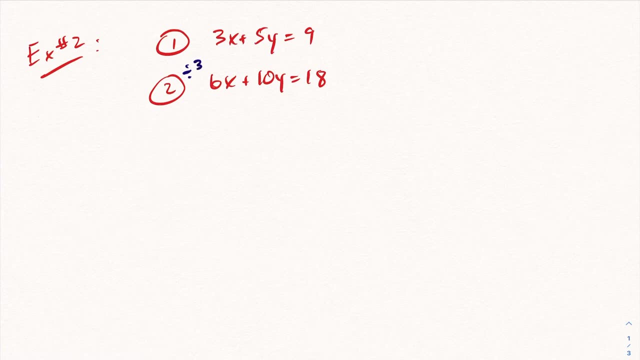 Well, quickly for equation 2, I can see I can divide across by 2 here, And if I divide across by 2, my equation becomes 3x plus 5y is 9.. And we can quickly see here That both of these equations are the same. 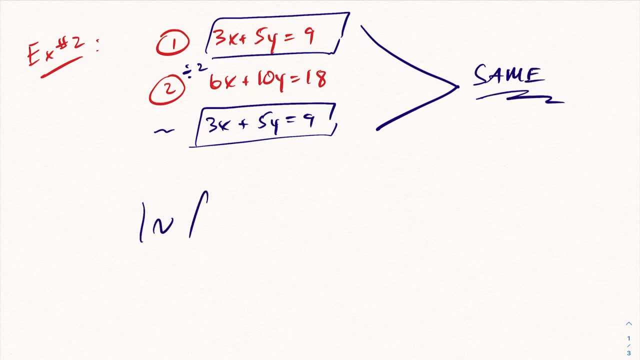 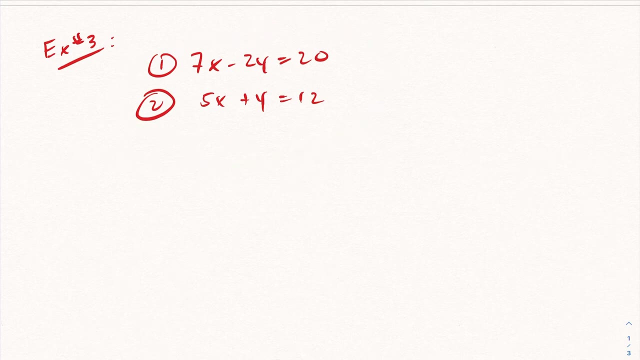 And because both these equations are the same, this would be infinite solution. All right. And example 3: here, Same deal. I don't see any way to reduce this right. I can't divide across by something, So the easiest way is to do a slope argument. 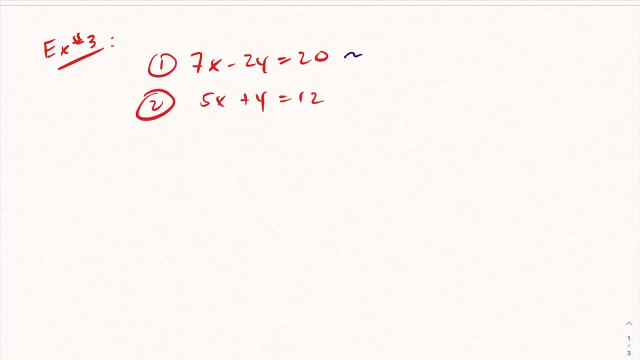 So one way you can do it is put this in the form: y equals mx plus b. So I'm going to try to isolate for y, Divide across by negative 2.. And I've got my one equation. Likewise, here I'm going to try to isolate for y. 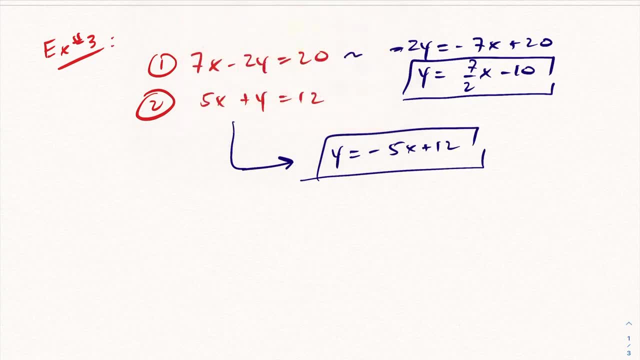 And we are in a slope-intercept form. So right away, as soon as I see this, with this equation here one slope is 7 halves, the other slope is negative 5. As soon as you have that, you can say different slopes and therefore unique solution. 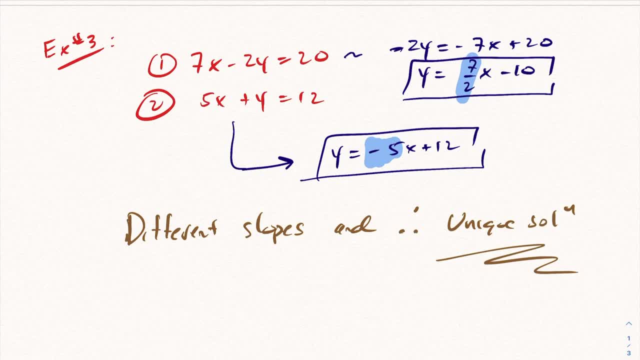 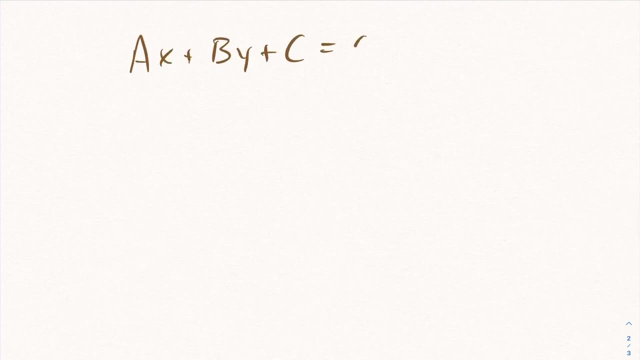 or exactly one solution. Okay, Just as a tip here, if you're trying to find the slope over linear equation, you don't always have to put it in the form y equals mx plus b, So like, let's say, in general you have general linear equation.